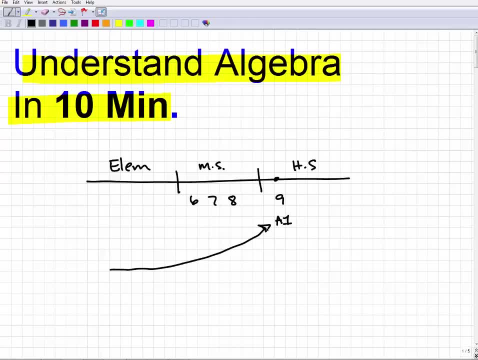 kind of ramping up slowly, slowly, slowly over your elementary school years, fifth grade, for third grade, fourth grade, etc. introducing maybe a little bit of concepts. you may not say you know that it's actually algebra, but in fact it is. and then in middle school you really start learning more and more algebra. 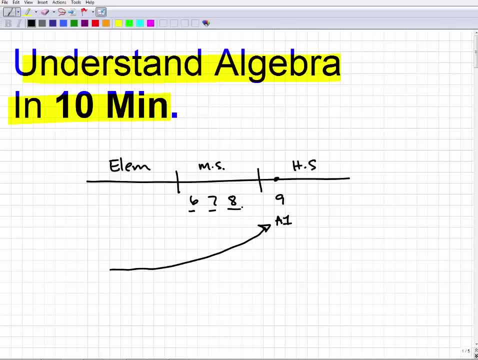 concepts: sixth grade, seventh grade, and then you- probably most eighth graders- are going to take what they call like a pre-algebra class. okay, even if they don't call it. so algebra is kind of this continuum, what's going on. so let me give you a. 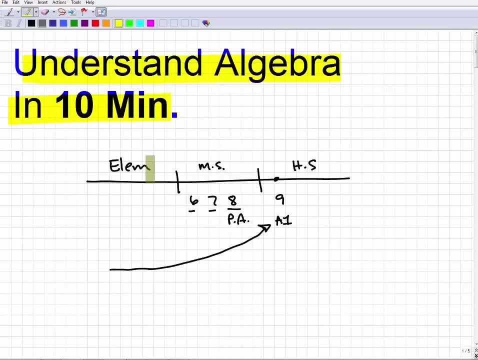 quick rundown here of elementary school. let's review this here, because in middle school you're kind of already learning algebra. it just may not be a full dedicated course, but in elementary school, remember what are you focused on here, what did you learn or what are you learning? typically, you're learning 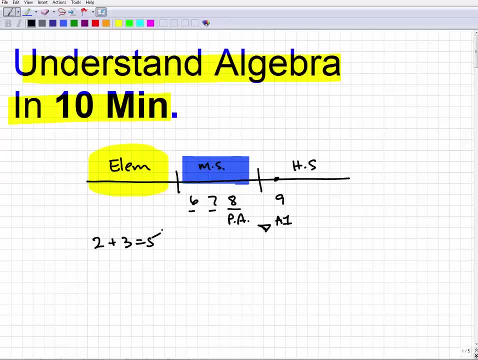 things like arithmetic. that is the main focus of elementary school. three times seven, one-fifth plus 2-7-th, how to handle problems like this division, three divided into 17, etc. so, and then your elementary school years. you're really learning a lot of arithmetic now. 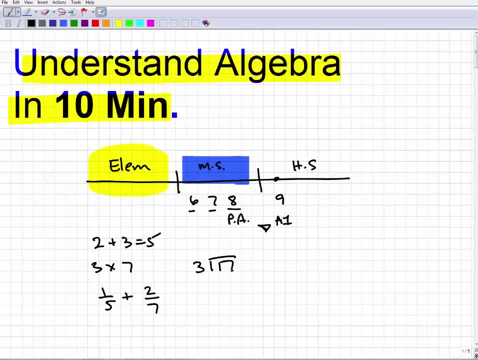 you might say: well, that's arithmetic. I want to know about algebra. the two are actually interlinked, so just you kind of follow me here in a second. so you spent a lot of time and effort learning about numbers and number operations, which is very important. in middle school we start kind of branching off and doing a 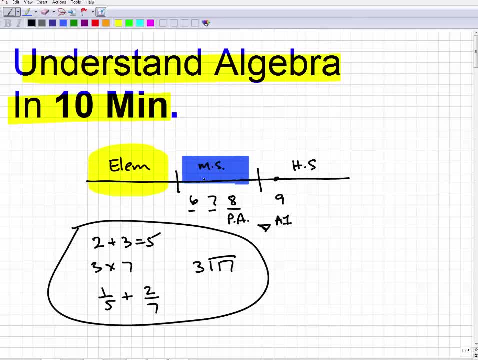 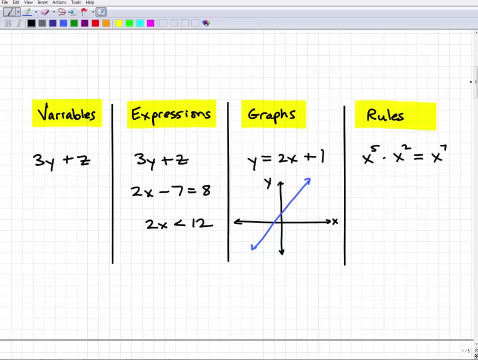 kind of transition into kind of a full-blown algebra course. so I'm gonna kind of outline with all that's about here in a second. so let's get right to it. and I kind of broke it up and in four main areas this is the way I'm gonna. 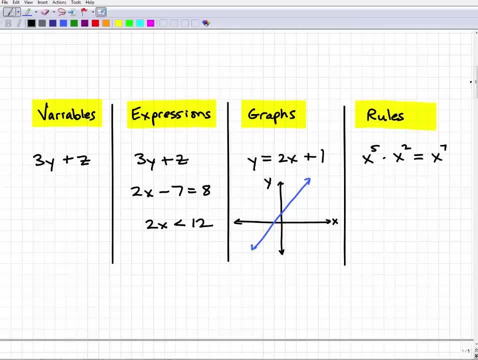 break it up. other people can break it up in various ways. you could break it up like the: like the chapters of a course that's too kind of narrow for the purpose of this video. I just want to give you kind of a big, global, big picture view of algebra, okay, so you kind of understand the essence of it. so an 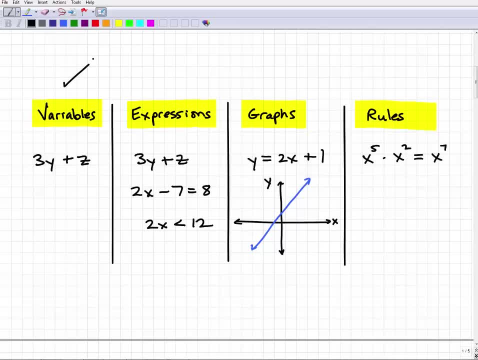 algebra. what's different from algebra, then, say arithmetic when we learned at elementary school years, is variables. we're working with variables, these things, these XYZ and all that kind of stuff, so we're really getting heavy duty into the use of variables in algebra. okay, I'll talk about more about each. 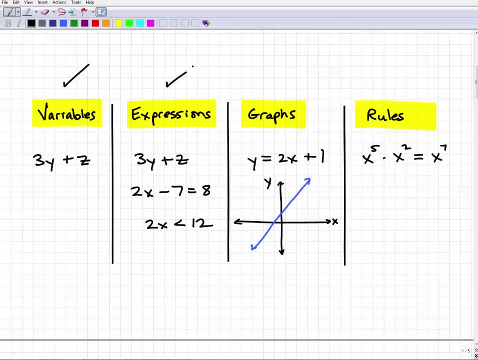 of these in a second. the next is expressions. now, expressions, this can mean a lot of different things. okay, this right here, this three Y plus Z, is something we would call to refer to as an expression, but in algebra we also deal with a lot of things like equations. equations, in fact, are a huge part of 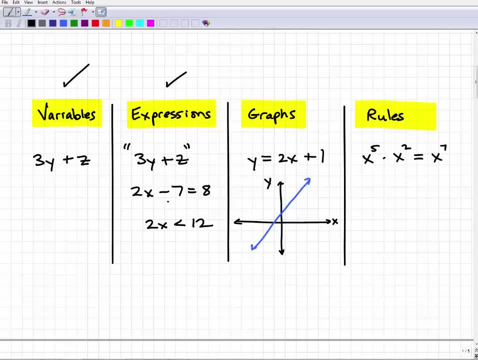 algebra again. I'm gonna get more into this in a second- and then we have these things like inequalities as well. so these are examples of the type of expressions that you're going to be studying in algebra now. another thing that you really get into in algebra is graphs, kind of in middle. 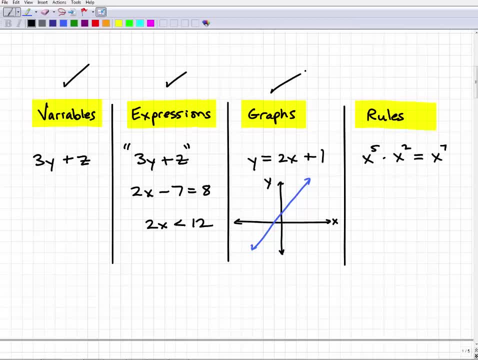 school and elementary school you learn kind of how to interpret graphs, but not so much the procedures to actually graph something. so we kind of really start this heavily in algebra one again in your middle school years and maybe previous years you've done a little bit of this, a little bit of that. 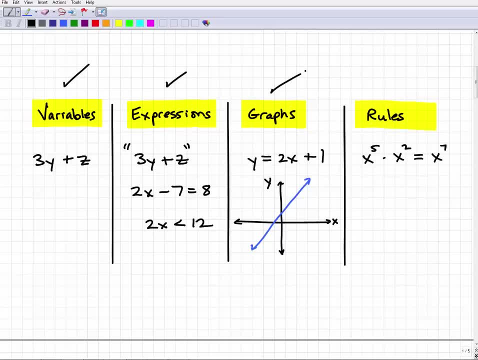 but in algerba one really start focusing on on graphs, because the graphical interpretation of an algebraic expression is very important. we need to be kind of, we need to be able to start to read the graphs, interpret the graphs, etc. so graphs in mathematics in general and I would say from algebra, algebra 1: 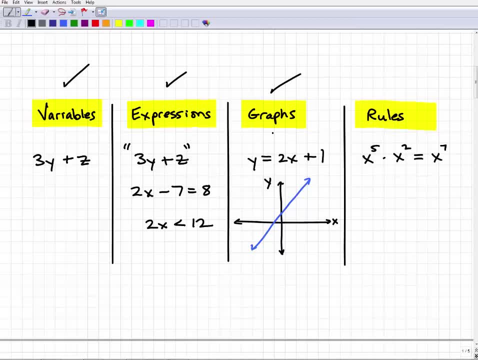 and beyond anything more advanced, is integral. so it's a huge part of what they're going to be learning and you're going to begin to learn a lot more in this algebra and then rules. okay, I break this up in my video. this could be known as: 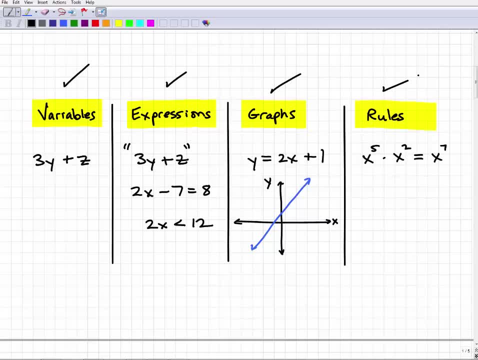 properties, rules, etc. well, there's a ton of little rules that you have to learn. this is an example of one. again, I'll get into this. okay so, variables, expressions, graphs and rules. in my view, this is kind of an kind of good overall view of what you're going to be seeing in algebra. okay, so let's get right to it. so 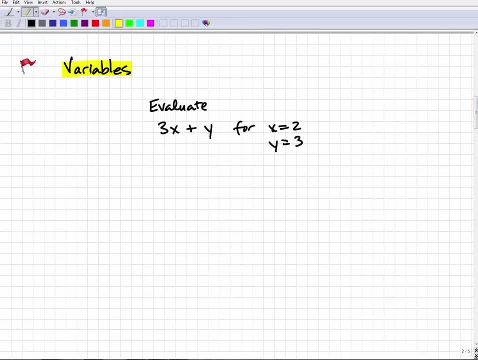 variables. all right. so what is a variable? if you don't know what a variable is? it's simply a letter or symbol that represents a number. that's it so. if I say X plus Y equals 7, well, X represents a number and Y represents another number. that's it so. and, by the way, because the symbols are, 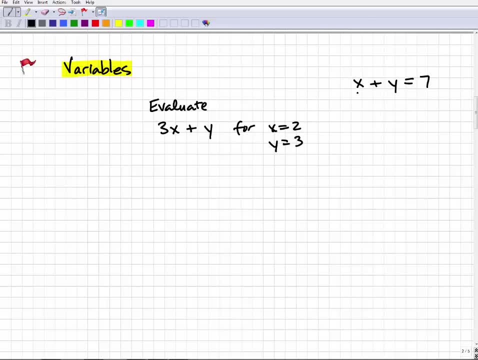 different: X and Y. I'm meaning that this is this number- is different than this number. so if I asked you what number plus another number, a different number would be equal to 7. well, we add them up, it would be 7, you would be like. well, 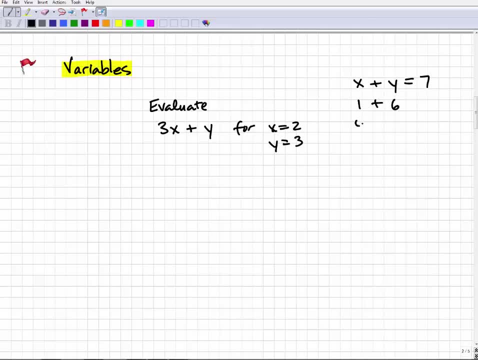 easy. that could be like 1 plus 6, or maybe 4 plus 3, or maybe 2 plus 5, and you'd be correct. so X. okay, we could say, hmm, this could represent any one of these numbers. and why I could any one of these numbers? These variables are nothing more than. 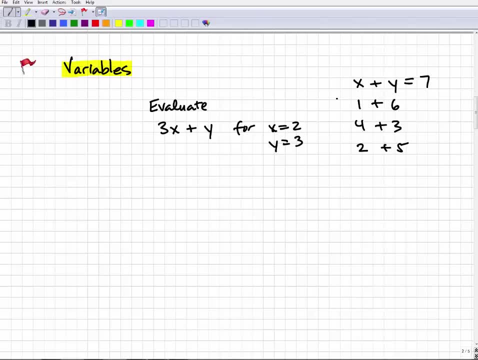 placeholders. So if you think back to your elementary school years, you might have seen a problem like this. This is something maybe you do like in, say, second grade They'd have like a little box and then it would be like plus two equals three. 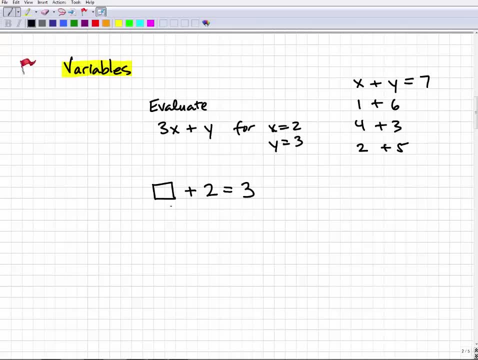 So this may be in first grade. So your student's looking at this. okay, what should I put in the box in order for this to be true? They're thinking about it. oh, okay, I put a one in there. Well, the box. 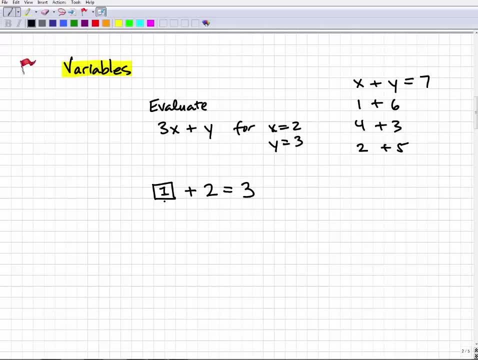 represents a number. In fact it is a variable. So variables are a huge part of the language of algebra. It is the language of algebra. It's what we're going to start really getting into in more advanced math, So you learn rules with variables, For example. 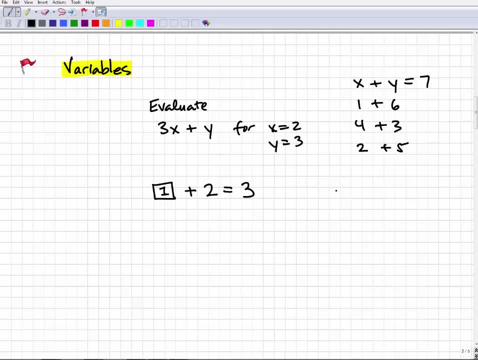 in arithmetic in your elementary years. you might say multiplication like: oh, three times two, that's equal to six. Or you might write it this way: three times two, that's equal to six, Or three times two, that's equal to six. But when 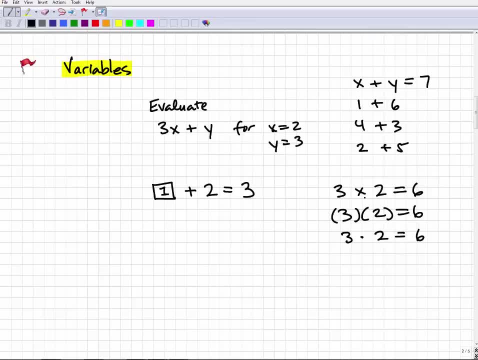 we use variables, we don't use these, this format here. okay, So if I have one number and another number and I want to say that I want to multiply them together, I simply write the variables. or sorry, one variable and another variable. I simply write the variables next to one another. 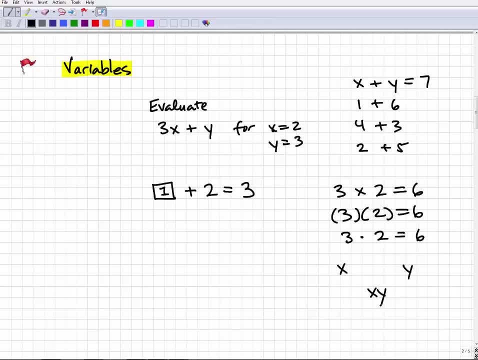 That means multiplication. So part of when you learn algebra and about variables, this is kind of some of the general format formatting rules of working with variables. Okay, so variables. Now, one of the things I really want to make clear is everything you learn back when you're in elementary school. 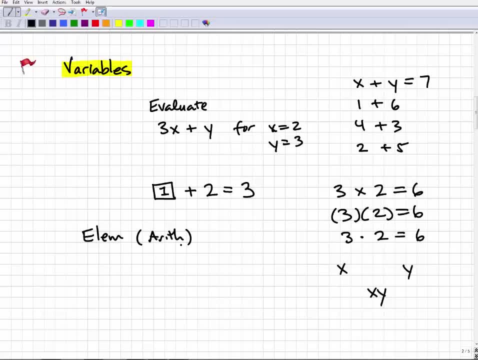 okay, all your arithmetic, you're going to follow those same rules. So you'll follow the same rules of arithmetic with algebra because we're using variables. Okay, so variables are nothing but more than numbers. But the rules to deal with number operations you learn back in arithmetic. 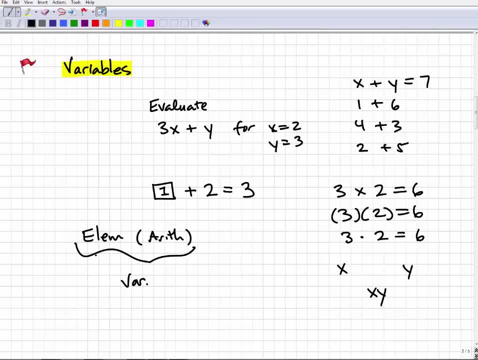 Okay, those still carry forward. So when you're manipulating or you're working with these variables, you have to think back. okay, you know, this means you know addition, this means you know multiplication, and you still have to use the same. 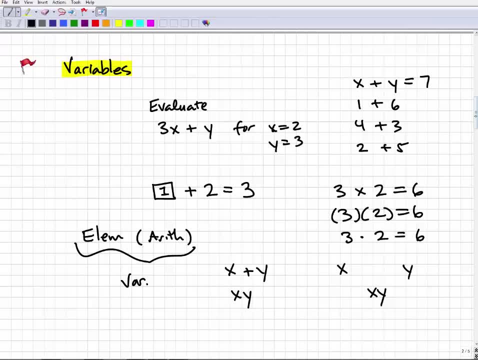 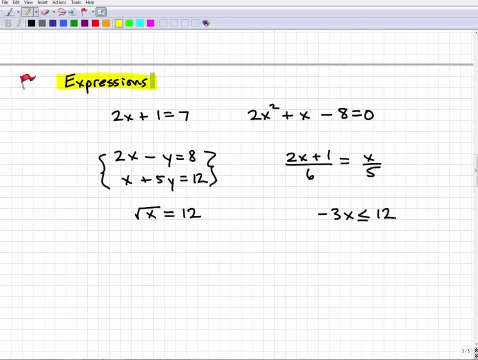 order of operations. Okay, so that's variables. Let's get into the next big topic here, and that is expressions. Again, the purpose of this video is just to familiarize you with a lot of what you're going to see in algebra. 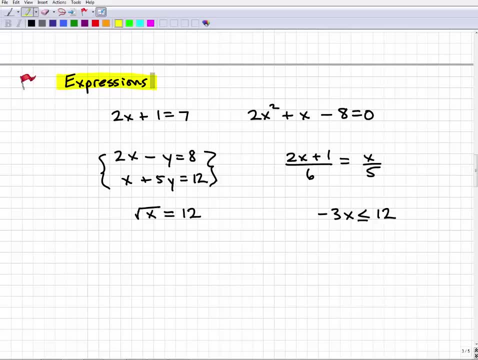 and kind of maybe demystify where it's not. It's not so intimidating, Okay, it's not. it's a lot you have to learn, but if you break it up in little chunks it does make sense. And again, the purpose of this video is to kind of paint a bigger 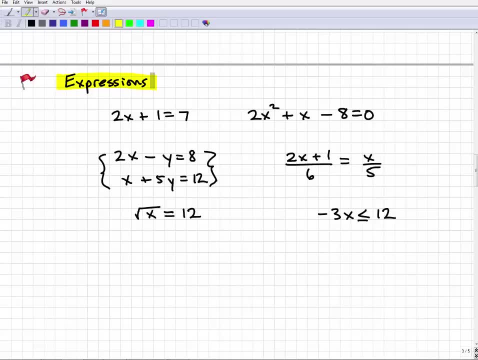 picture for what you would see in this course. All right, so expressions. Well, I would say by far the number one type of expression you're going to be studying in algebra are equations, okay, statements with this little equal sign. These are various examples of some of the type of equations that you would see. 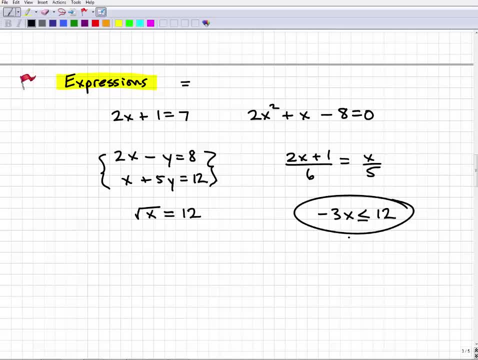 This guy over here. this happens to be an inequality. We'll talk about this in a second. Okay, so equations. let's kind of go down here and just talk about what an equation means. Okay, so I have here: 2x equals 8.. 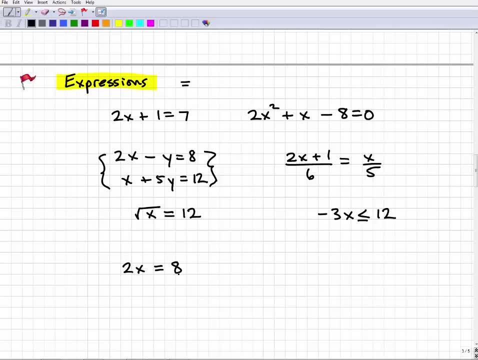 All right. so this is a basic equation. An equation is they almost kind of think of it as a question. It's saying hey, 2x. remember, in algebra talk this means 2 times a number, some number, x. okay. 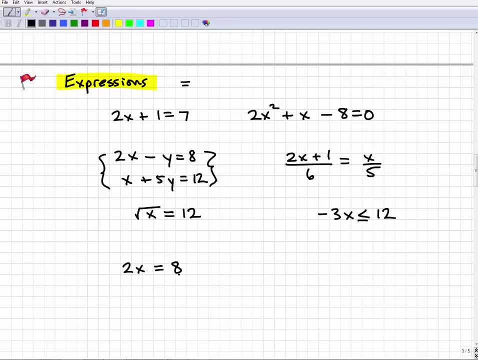 So 2 times some number, x is equal to 8.. So if I asked you just right off the bat, hey, 2 times, what is 2 times 2 times, what number is 8?? Well you would be like, oh, that number is 4, okay. 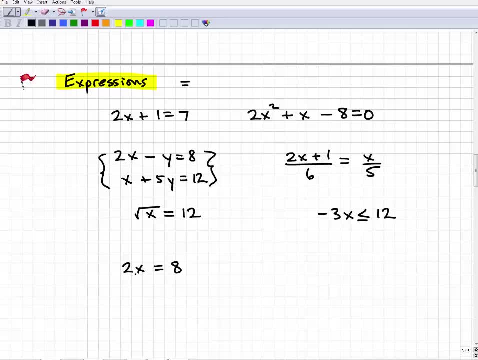 Well, here the idea is to solve these equations, to find the value of this variable or variables such that it makes this statement true. Okay, so if I substituted a 4 for this x, I would get 2 times 4 is 8, and 8 equals 8 is true. 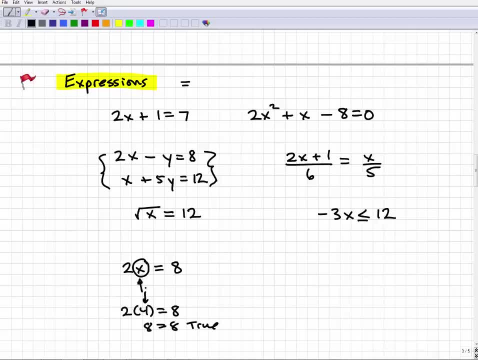 Okay, so the number that we plug in or substitute for the variable is what we call the solution. So we're always looking for solutions in algebra. It's the number or numbers, depending on how many variables you plug in, such that when we replace the variable with the actual number, 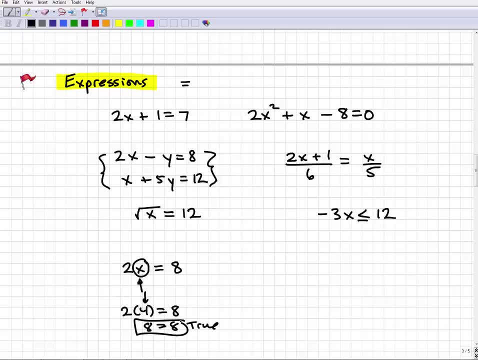 it balances out The left and right hand side. the left to right hand side of the equation is in fact true. okay then, in other words, of the same value. that's the whole idea of an equation, so it's kind of like a riddle or a challenge. hey, find that number that. 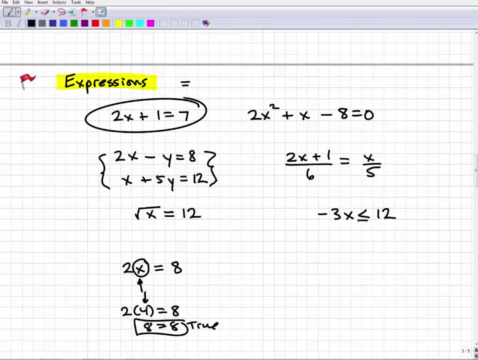 makes this true. so let's take a look at this guy here real quick. okay, so two times what number plus one is equal to seven. just think about that for a moment. what is that number? okay, what's this number here? two times what number plus one is equal to seven. even if you've never taken any algebra, just kind of try. 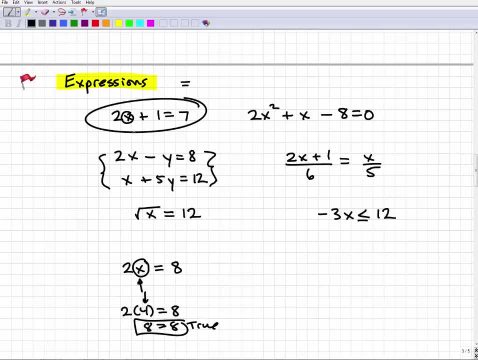 to reason that out. alright, so hopefully you determine: and that is 3, okay, so 2 times 3- it's kind of right here- plus 1 is equal to 7. 2 times 3 is 6. okay, it gives me a 6 here, and if I add a 1 to it I'm gonna get 7. so 3 is. 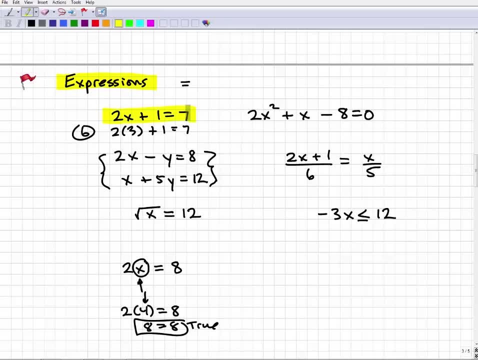 it and the other number. please take a look at that. it gives me a 6. it's 6 plus 1 is equal to 7. so the answer is 3 plus 1 plus 1 is equal to 6 plus 1 is the solution to this equation. okay, now, this is a particular type of equation. 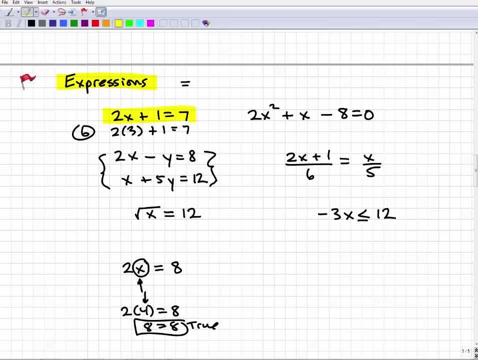 something we call a linear equation. so in algebra we're going to learn the different techniques to solve on your equation, and it's just a bunch of methods, okay, so think of it as a kind of little computer program or recipe. you go into your kitchen you say: bake a cake, you got to do, you got to do this, you got to do. 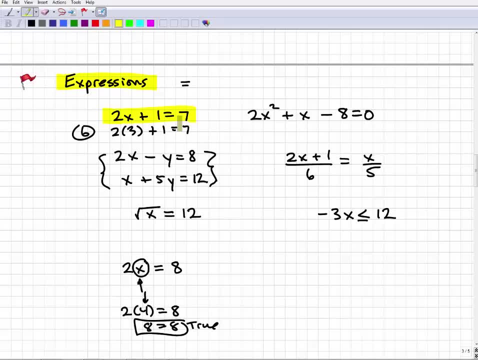 that you got to get this, you got to do that. algebra is very much that way. it's very procedural. okay, I'm gonna give you a set procedure, okay, to kind of follow through. if you follow this procedure, you'll get the solution. it's very methodical. so it's not like, let's say, creative in terms of like, well, I gotta. 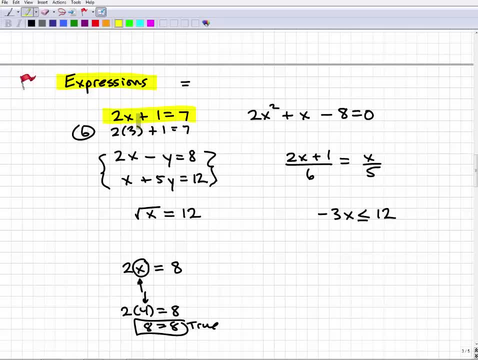 go find I got to create a way, a new technique. no, it's just a procedure that you have to learn and practice. okay now, this is a linear equation and in algebra- but in algebra especially up to the Algebra 1 level- you're gonna be studying different types of equations. so here are some other. 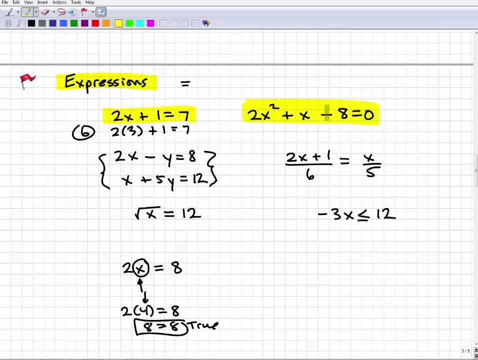 examples. this guy over here happens to be a quadratic equation- okay, you notice it's different- has a next squared. this actually has two solutions, not just one. this guy had one solution. right, an equation like this would have two solutions. so we have to learn the various technique, techniques and methods. 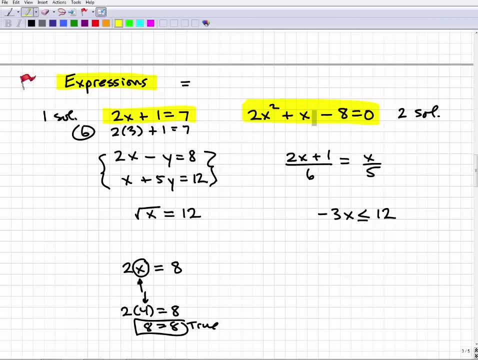 and they're, you know, considerable. they're a good amount of things you actually do have to learn in order to solve an equation like this. not overly complex, but things that we, you have to study and and focus on to to get this down okay. this type of equation is totally 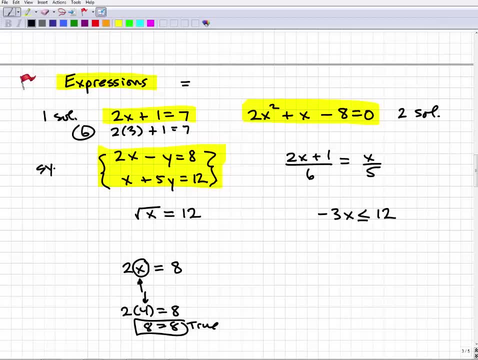 different. this is something we called a system. okay, again, it's a type of equation. this is a system of linear equations. okay, so we have this equal sign. so we're still looking for numbers for X and Y, so we plug them in. it's gonna make this, these equations, true. okay, you're gonna. 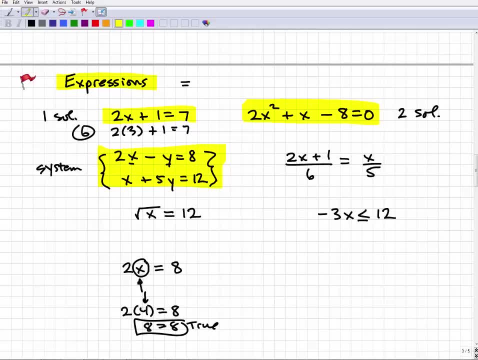 learn a lot about systems in algebra- a huge topic. now here's another type of equation. okay, this is a rational equation. this particular one is also referred to as a proportion. okay, so you're gonna learn other rules, but again, we're still looking for the values of the variable that makes the the left. 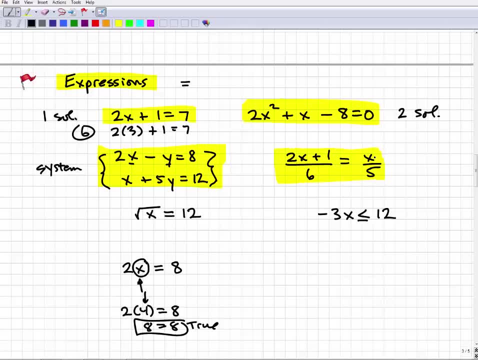 hand side equal the right hand side. so equations are huge. huge part of algebra, huge part okay, and there's more down here. forgot about this guy. this is a radical equation, okay. so if I plug in the square root of what number is gonna equal to 12 again? 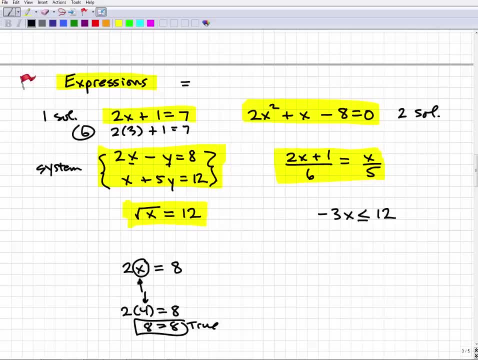 there's various techniques and a lot of it is pattern recognition. when I see this type of equation, I'm going to use this method. okay, I use this procedure. when I see this type of equation, I'm going to use this procedure. when I see this type of equation, which is called a system, you're going to use this. 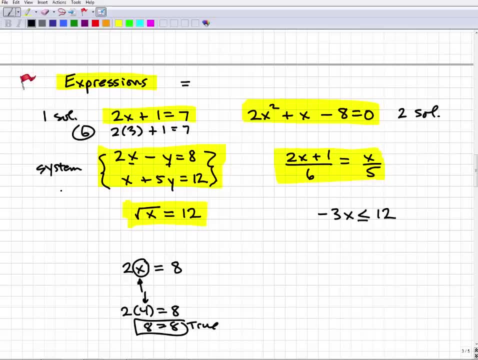 this, etc. okay, now, as you become more advanced as a student, you'll learn more and more about the characteristics of these equations. you can learn more about what they mean, the properties, you go more in depth. but as a math teacher myself, my first goal- and probably most teachers goals, is to get you to, to. 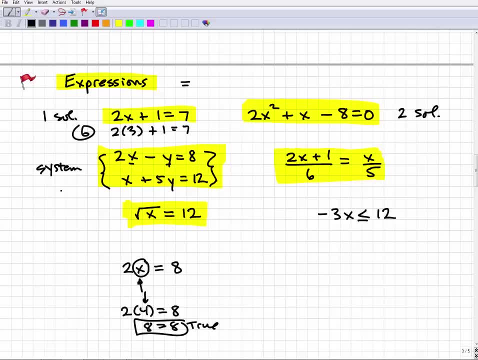 master the, the actual practical procedures to solve these equations. okay, that's a huge part of it. okay, you'll, as you study math, like I said, you'll learn more about them and, trust me, that's a big topic. you can get into very detail and you will, as you continue to study math, algebra to precalculus, you'll get. 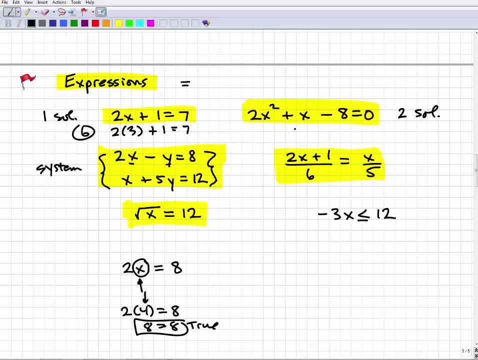 into much more detail about what these equations mean. okay, for example, this guy over here is that happens to be a, also a polynomial, and there's different things you want to know about polynomials. that's a huge topic in algebra, but again, this particular video is focused on this particular topic and I'm not going to 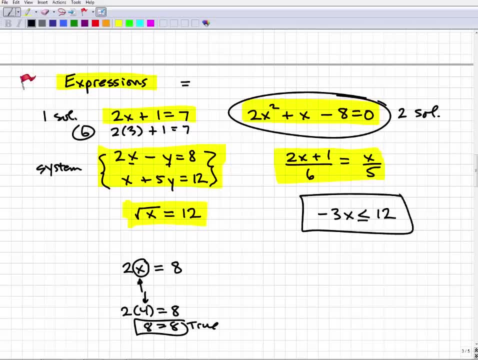 focus more for the algebra, one level. now let's talk about this guy real quick. this is an inequality, okay. so an inequality is: is those signs right here, like less than or equal to, greater than or equal to, etc. I'm giving an easy example: if I have, X is less than 7, okay, what would be a solution? okay, what? 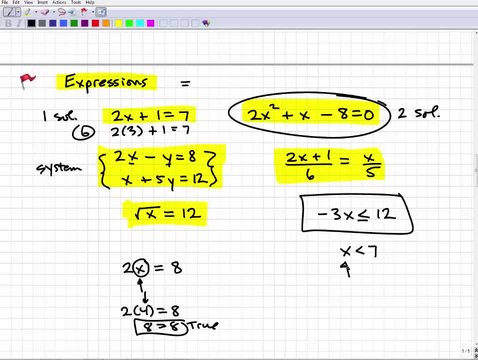 number. can I substitute for X? that would make this true. so let me ask you, what number is less than 7? well, you probably said six. okay, six is less than seven. that's true. okay, that's that, and that would be correct. okay, but that's not the only number. okay, so it was five. five is less. 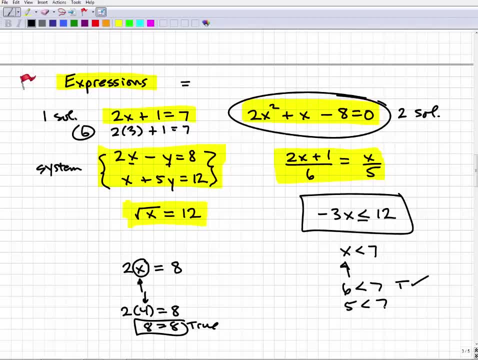 than seven. four is less than seven. there's actually infinite amount of numbers that are less than seven. so inequalities are another topic that we study in algebra. they're very they're similar to equations and in that we use a lot of the same kind of procedures to solve them, but they're different in terms. 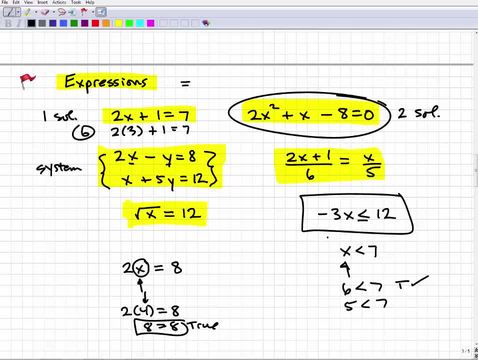 of their equations. but this is something that you're definitely going to be learning in algebra and, again, you probably have already seen some of this, for sure, in your elementary years and middle school, etc. but in algebra one you're really going to get into the procedures to solve full-on in the 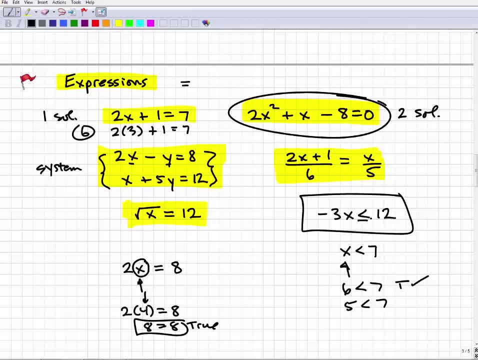 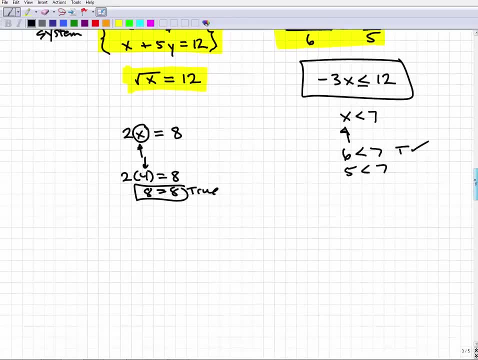 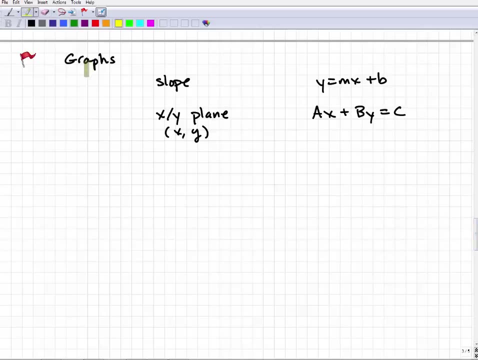 qualities, okay, and there's different type of inequalities, linear inequalities, compounding qualities, etc. but this is a little subtopic, that's within algebra. okay, let's go ahead and look at the next slide. let's move on to graphs. okay, so graphs, another big, huge area of algebra. okay, as. 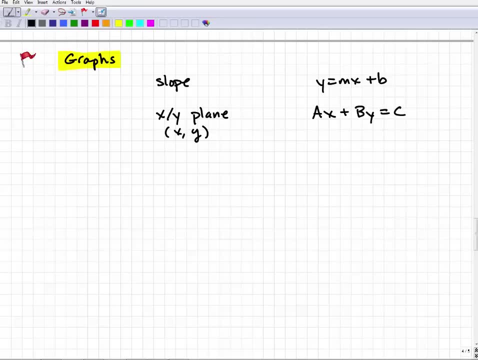 I was telling you back in your elementary school days and middle school days we did a lot. you probably did a lot of interpretation of graphs like bar graphs or or pie graphs, just looking at them and kind of getting a visual perception what they are. but in algebra one really want to start taking various 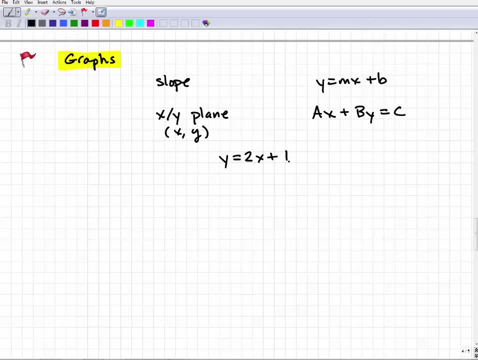 equations okay, maybe something like this. and looking at its graphical representation, okay. so here I have an equation. sometimes equations, okay, we can also think of these guys as what we call functions. all right, and I didn't put this down as one of the main areas of algebra, one, but it is a huge area- a function there's. 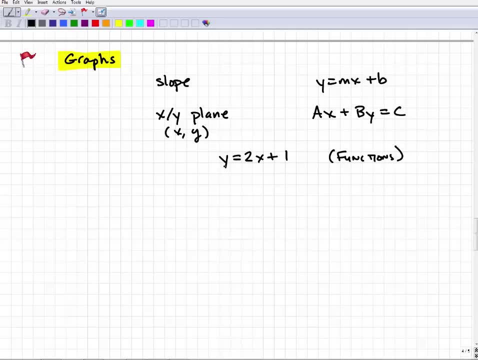 nothing more than an equation, okay, something like this, but instead of having this Y here, we put this little symbol, a f of X. it means the same thing. okay, so this is a linear equation and this is a linear function. now, functions have their own kind of concepts involved. okay, very. 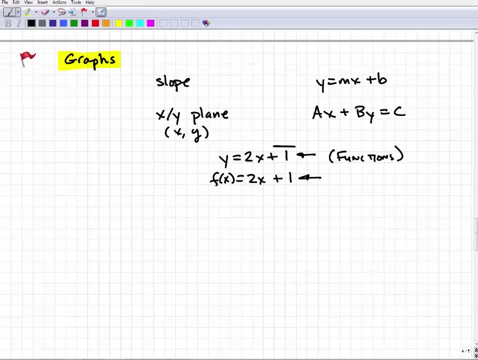 very important in terms of algebra, but we kind of treat them similar, similarly when we're talking about graphs. okay, so again, I'm not trying to teach you every single thing that you're going to see in algebra, one just trying to give you the bigger picture. so let's talk about graphs real quick. so in graphs, kind of 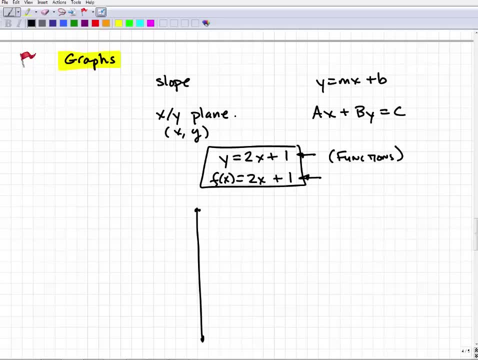 wrote different things up here. you're gonna learn about the slope and the XY plane and different formats of lines etc. so I'm just gonna just very quickly lay out some things here. what I'm drawing here, sketching out, is a basic XY coordinate plane. most you've probably already seen it. if you haven't, all it is. 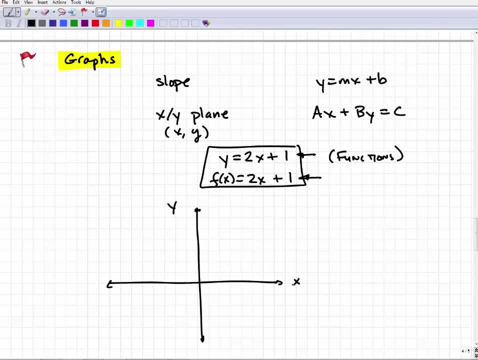 is basically like a mapping system, a coordinate system, okay, and we put a little points down on this plot, this chart and in the Y D. here is we. we have a system to to plot points and other and and graphs. okay, so the way it works is we? 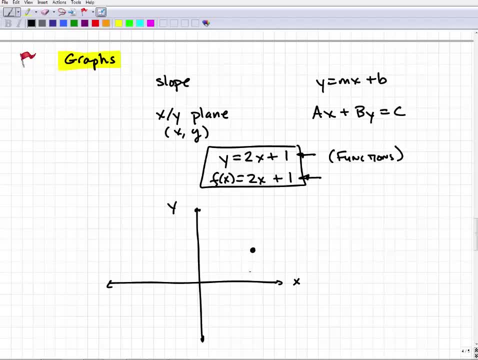 have an x-axis and a y-axis and we kind of it's a grid system. so, like this point here, we're good. I'm gonna go in and give you the location of that point, then I'll explain to you what it is okay. first I'm going to count on the x-axis, one, two. 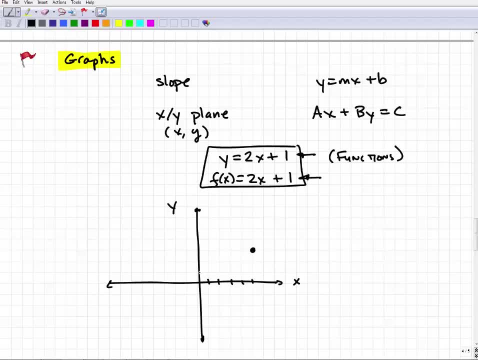 three, four, five. so that's five on x-axis and it's one, two, three on the y-axis. okay, so to describe this point, we always put the X number first and the Y number second. that's something called. we call an ordered pair. it's gonna be a. 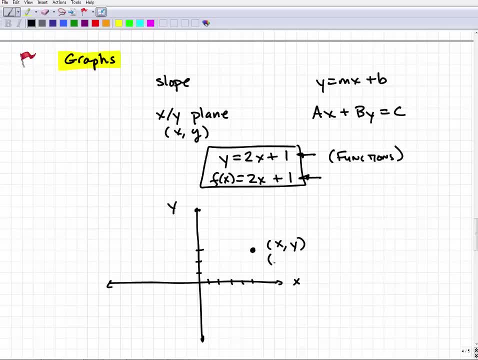 pair of numbers in a particular order. so this point is located at five three. it's no more difficult than that. okay, now here we have various quadrants. this is the positive side. this is the negative side down here. negative, this direction again. I'm not going to try to teach you all of this, but just to kind. 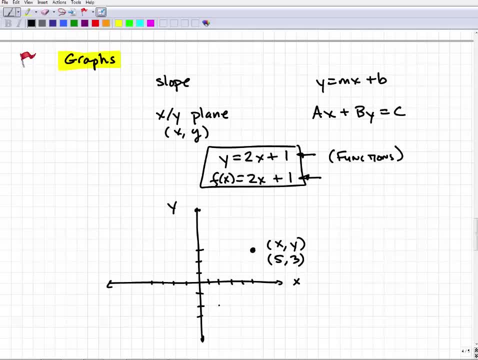 of indicate for you- those you've never taken algebra, that it's not that difficult. it's a basic, just kind of coordinate system. all right, an address system, if you will, for points. now I can have this point, and if I had another point, let's put a point down here. if I had two points and I connected those two, 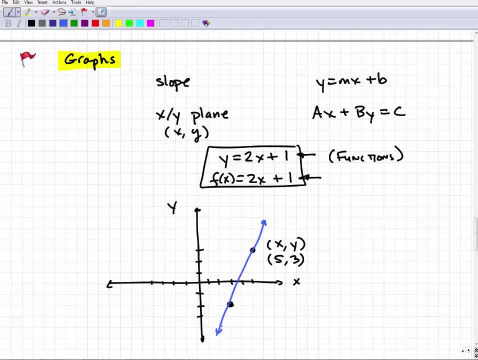 points here I would have a line, okay. so the way we graph lines is to basically determine two points that are on that line. okay, and this is one main technique, two points that are on that line, and then we just draw a line through it. so being able to graph lines is a huge part of algebra. now you're not only gonna be. 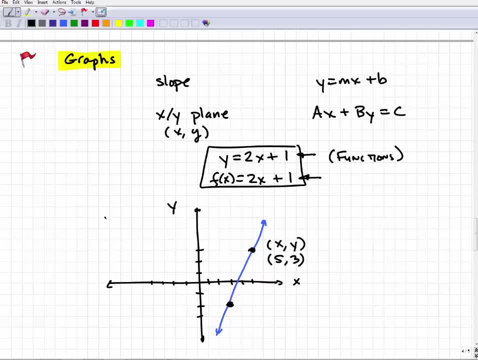 graphing lines. you're gonna be doing other shapes as well, okay, so you're gonna be doing things like u-shaped type of graphs. those are called parabolas, so you'll a big part of we're gonna be doing this lines, but you're gonna also be 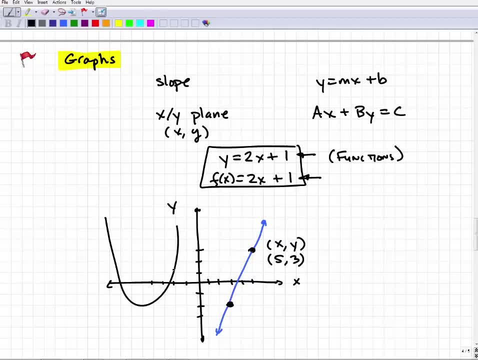 introduced to other different types of shapes- again, not as difficult as you think, but it's all done on this kind of XY coordinate plane. okay, now you're also going to be asked to find the equation of a line. so for example: hey, I have a line that goes through these two points. give me the equation of that line, okay. 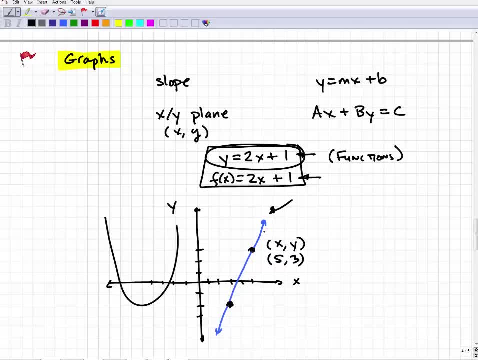 so, for example, this line here I can actually plot like I have this blue line here. okay, I give you the equation, you give me the line. but a big part of algebra is: I'm gonna give you the line and I want the equation back, so you're gonna have. 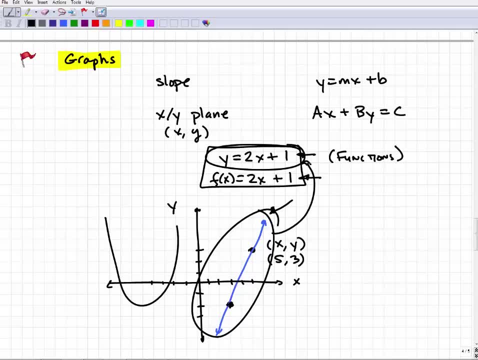 to go in both directions. okay, so that's a good, good chunk of what you're gonna be doing in algebra and it's as necessary kind of you know study, because in more advanced mathematics you're gonna see how graphs are gonna be key. you're gonna be doing lots and lots of graphs for those. you're out there, that. 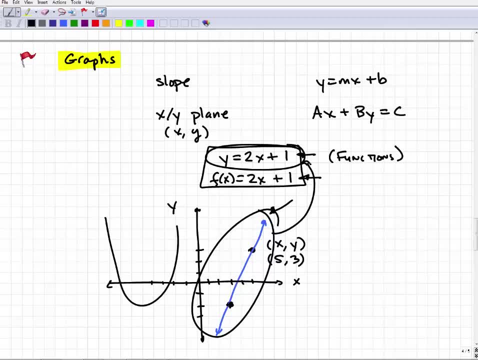 are going to be going to say precalculus, you're gonna be doing trigonometry, a huge amounts of graphs, or you're doing things like conic sections. if you've done that, you can appreciate what I'm saying. you're gonna be learning how to. 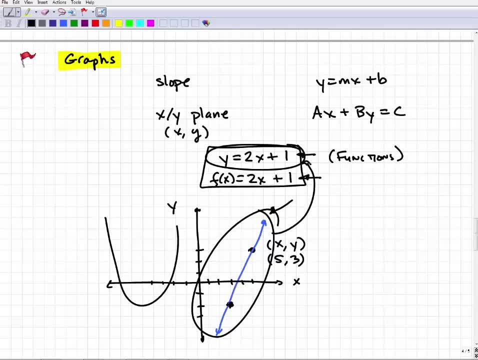 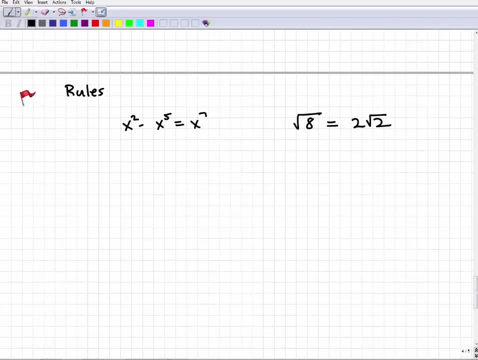 do tons and tons of graphs, but this is where your first kind of real introduction to to learning how to graph, learning this XY plane etc. happens in algebra one. okay, let's move down to our last thing, and that's I'm gonna call rules. we can call this rules, procedures, properties, etc. but there's a lot of things we just 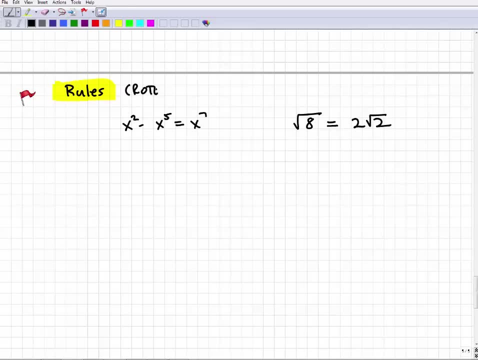 need to kind of know. they're good old-fashioned rote memory, or wrote me. if you don't know what memory is, that's simply just kind of flashcard memory. like you know. if you remember how you learn your times tables, you just kind of had to learn them. you had to go through the flashcards until you finally got. 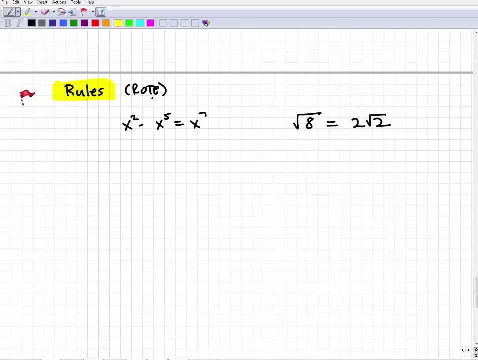 them down. same type of thing in algebra: there's a lot of rules that you're gonna have to learn more about than you're just going to have to learn them. okay, so get yourself some flashcards, etc. here. here's one type of rule. okay, this is has to deal with with powers and properties. now I can teach. 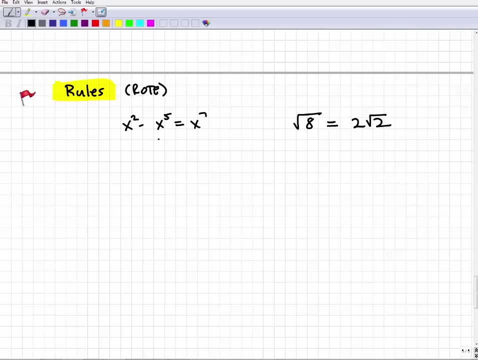 this to you in a way where you'd be like, well, I don't need the role because I can separately kind of understand what's going on, and that's fine as well. but most students will be given a rule something like this: a to the M times a. 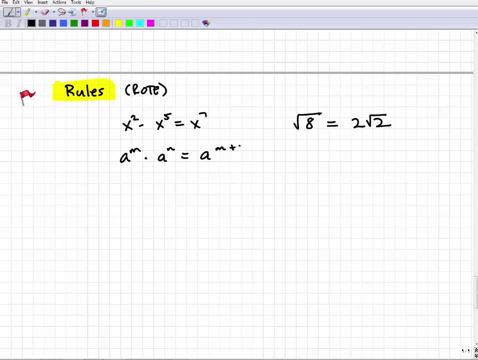 to the end is equal to a to the m plus n. so this is a particular rule and you can rule that you're going to have to learn. So in algebra we're given these rules okay. Then we're given various examples of how to apply the rules. okay, And I would say there's a pretty good. 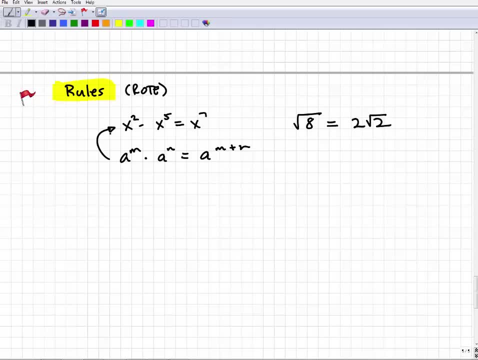 amount of that in algebra one- Again not overly difficult. Even this particular rule here has to do with the multiplication of powers. I'm not going to get into all of it, but it's not that difficult, okay. It's just a lot of rules that you have to learn, So I think that's part of what 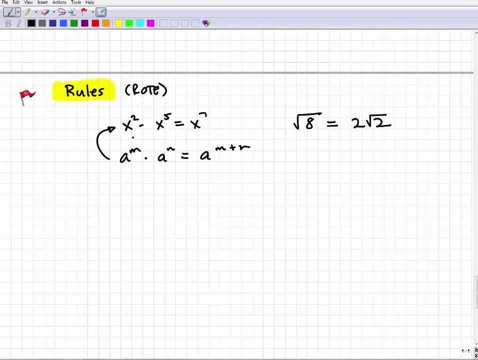 a lot of students struggle with in algebra. They get overwhelmed by not so much the complexity, just by the amount of stuff they kind of have to remember, And that's understandable. So my advice to you is: take great notes if you're taking algebra, and do a lot of review, A lot of review. 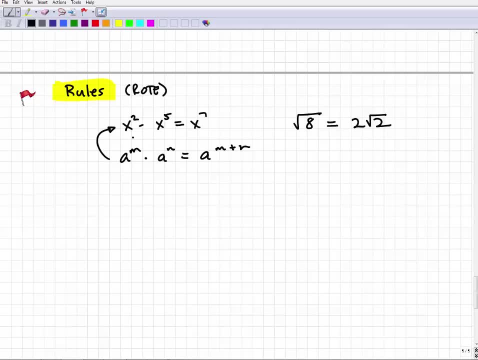 and you know understand those more basic level problems, because the more challenging problems are going to you know are going to challenge you. You're going to get frustrated if you're like, oh, I don't get this. Well, if you didn't get the more basic problems first, then you're never going. 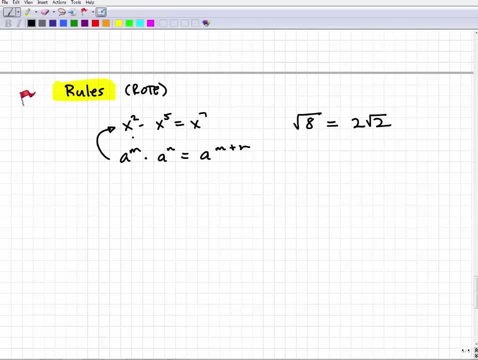 to be able to do the more advanced problems And you're going to be doing. you're going to have to do the advanced problems to pass your course. It just makes sense, right? So lots of rules and lots of properties when we're talking about solving equations, procedures and things like that. 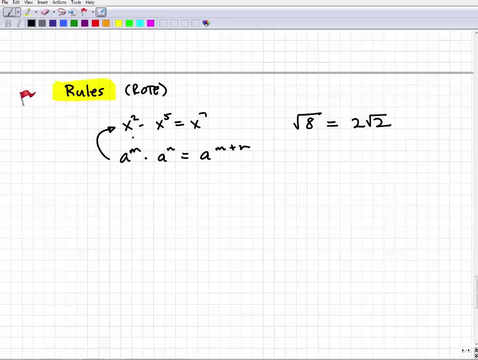 But nothing that you can't get through. Really, it's about your study habits. This is a huge indicator. Again, I'm going to hit this for you students out there: If you're struggling with algebra, I can almost guarantee you that your study habits aren't where they need to be In. 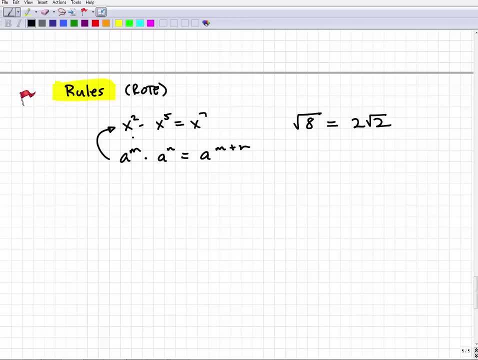 other words, you're not writing neat, Okay, you're not taking good notes, You're not showing all your steps. You need to try to model your work like your teacher is doing. Okay, that will help you tremendously. And over here here's another one. So if you're struggling with algebra, you can 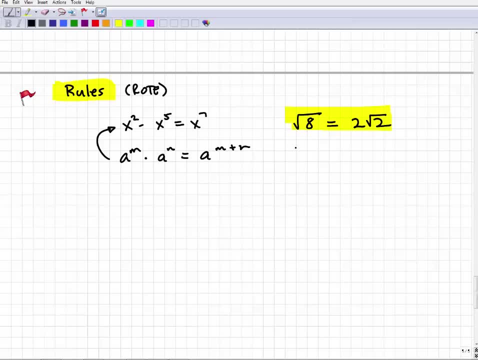 do this. This is another kind of example. If I give you the square root of eight, we have to understand what this means. Okay, and there's rules and things, how we simplify expressions like this. This is not an actual rule, but there is procedures involved. Okay, rules, properties. 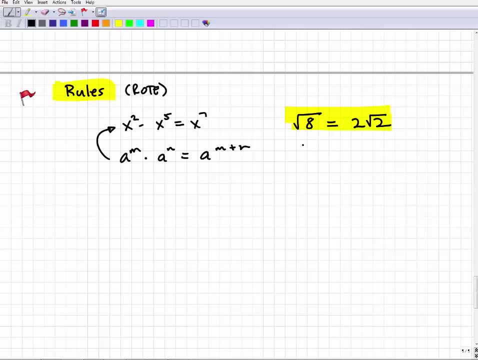 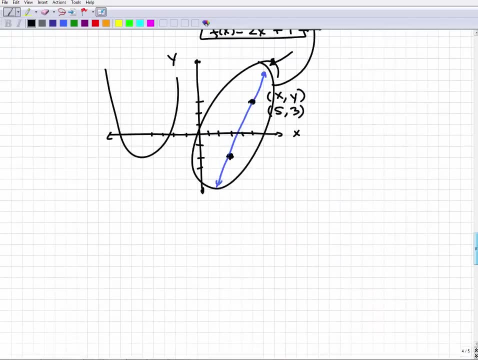 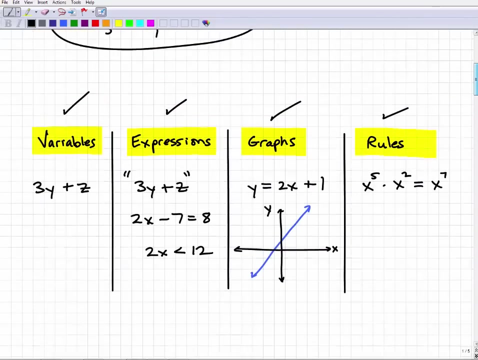 procedures, a lot of that in algebra one and in mathematics in general. But I can tell you right now, algebra one, okay- or algebra in general, up to say the beginning of your highest school years, is really not much more than these. This right here paints a good global sense of 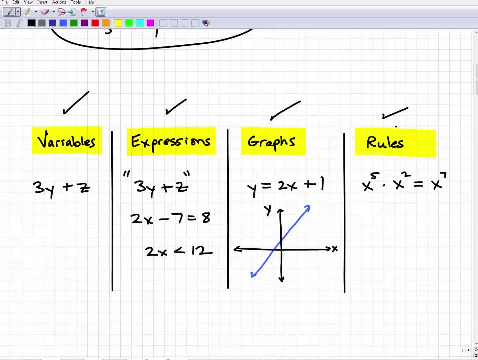 what's going on. There is a lot of little things in there that I didn't put. Of course I can't do all that And, by the way, I know this video went over 10 minutes, But if you understand what I was, 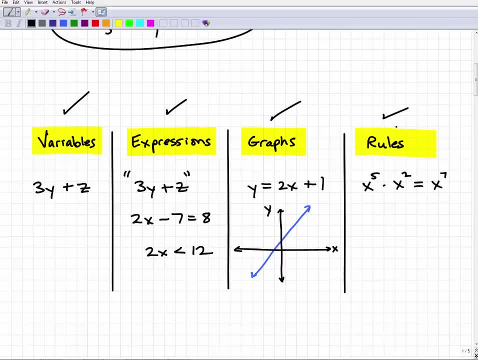 trying to say: here you're going to. you got a really good feel for what is expected of someone learning algebra. one okay, Like the end results. okay. Being able to handle expressions and with variables, understanding what they are, solving various types of equations and inequalities, being able to graph things. 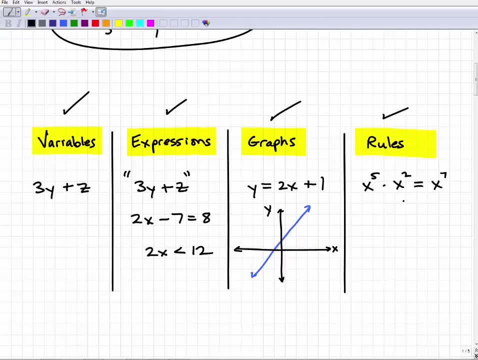 being able to find the equations of graphs and being able to recall lots of rules, procedures and properties, Just as you see something, a lot of. it's like pattern recognition too. Hey, I see this. God needed this particular rule. 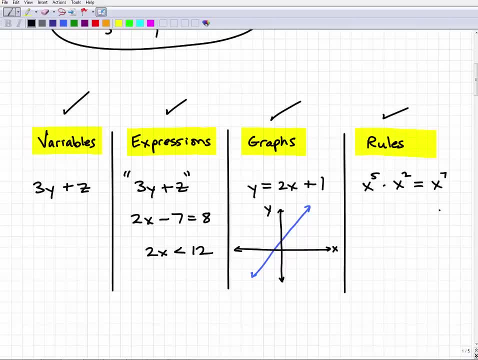 Again, a lot of teachers don't want you just to operate on rote memory. They want you to understand, fully comprehend, what that rule means. Well, I won't say this much As long as you could do the problem and solve it.